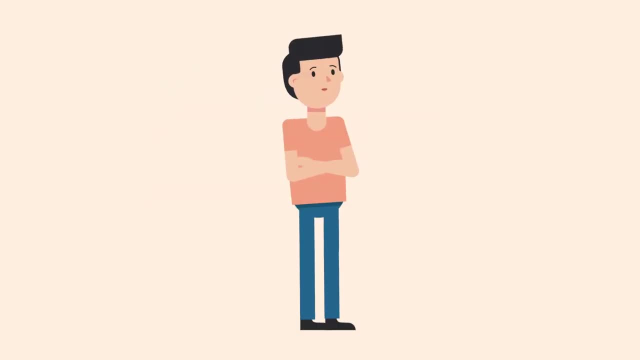 So you've been using Premiere Pro for a while and decided it's time to make an animated video. You see cool animated videos everywhere- Sales videos, explainer videos, training videos or YouTube videos- So of course, you want to make animations as well. They're awesome. 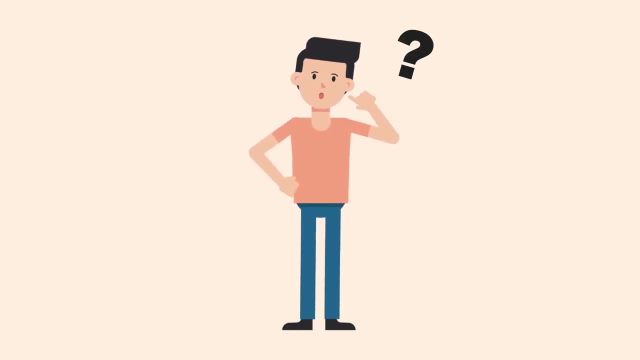 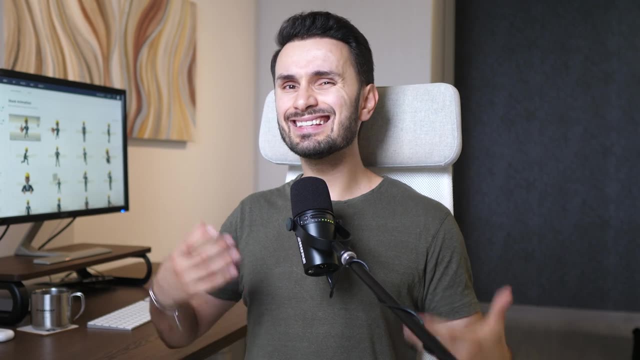 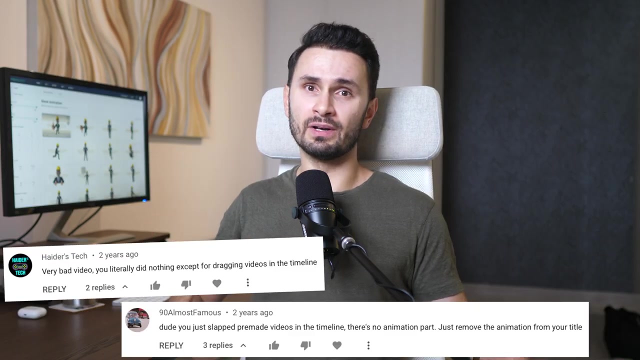 And you might be wondering: how can you make professionally looking animations in Premiere Pro? The problem is you've never produced any animated video before and it seems quite complex, So it's not very clear where to start. Now, before we get into it, I can already see the comments, so I want to address this up front. 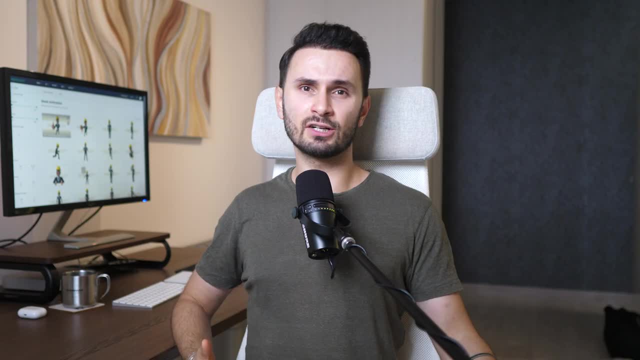 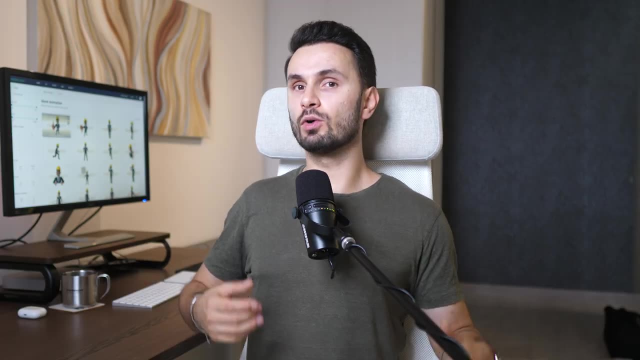 Oh, this is clickbait. Oh, I want to be a Pixar-level animator after watching a 7-minute YouTube video, and so on. If that's what you're looking for, no problem at all. But if you want to learn all the skills, you need to produce animations yourself. 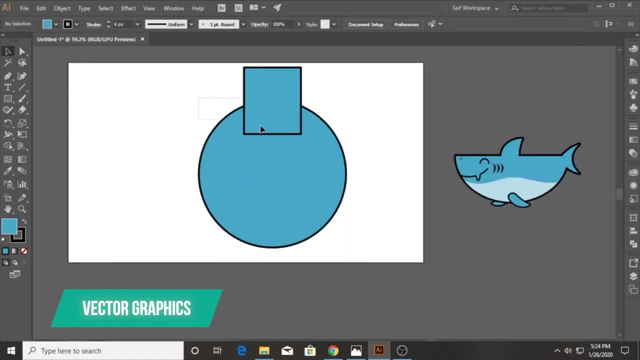 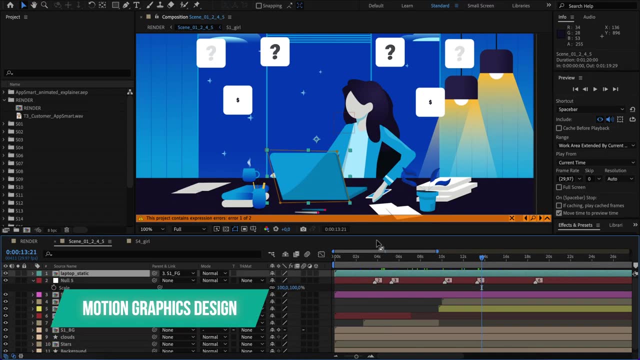 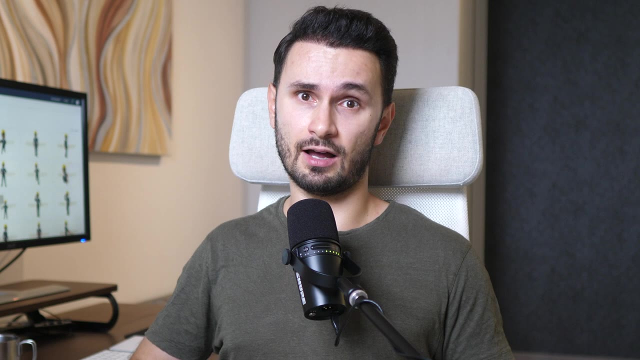 from scratch. that's a minimum of 1000 hours of training to get super good at that. Vector graphic design in Adobe Illustrator, motion graphic design in Adobe After Effects and character rigging using various plugins- Pretty complicated stuff Now. if you have the time and commitment to do all of that, that's great. But first, 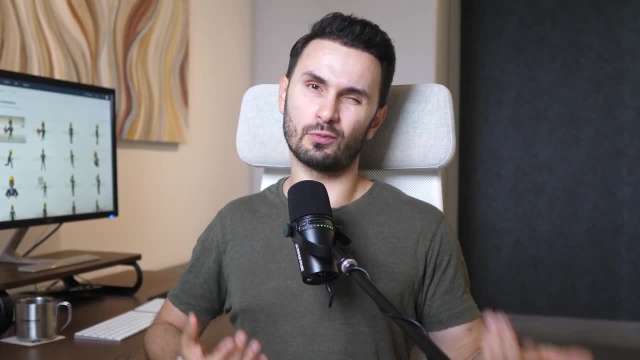 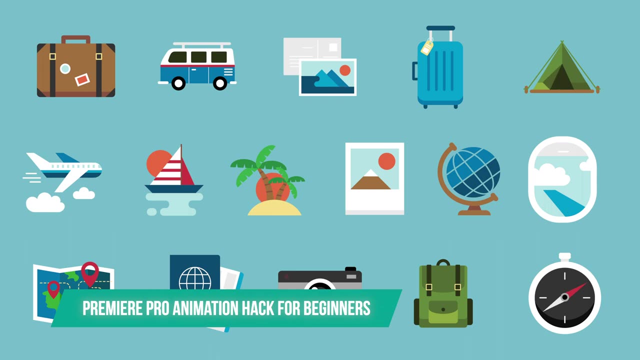 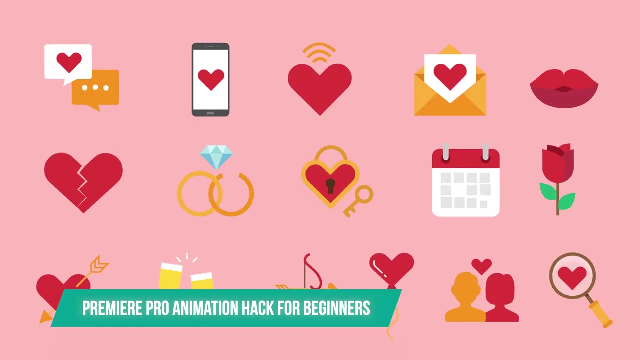 you will need other software, because that's impossible to do directly in Premiere Pro. And second, this is not a video for you, my friend. However, this is called a Premiere Pro Animation Hack for Beginners for a reason: Because what I want to show you is how to skip all the boring parts and achieve the same. 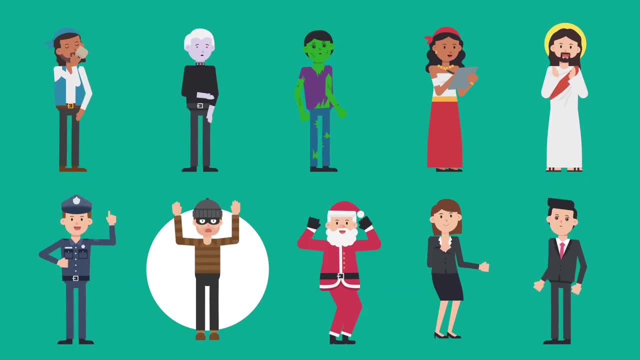 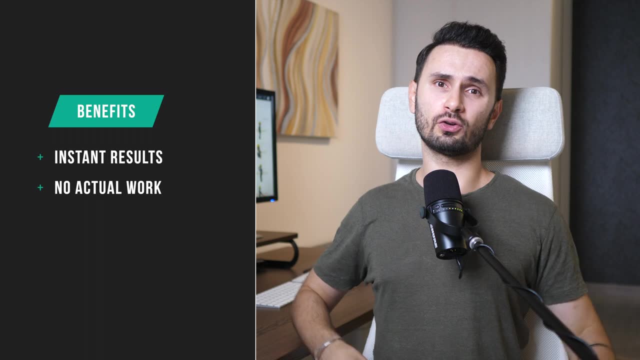 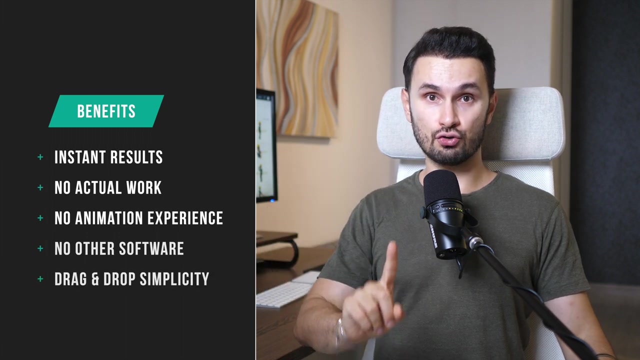 level of professionally looking animations directly in Premiere Pro. So if you want to have the exact same results instantly, right now, without all the hard work, without any animation skills or experience, without needing any other software, with literally drag and drop simplicity. 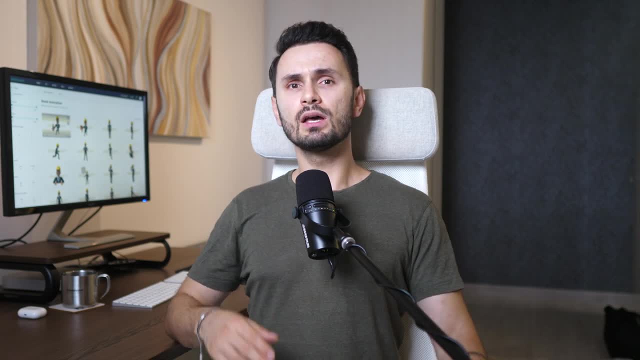 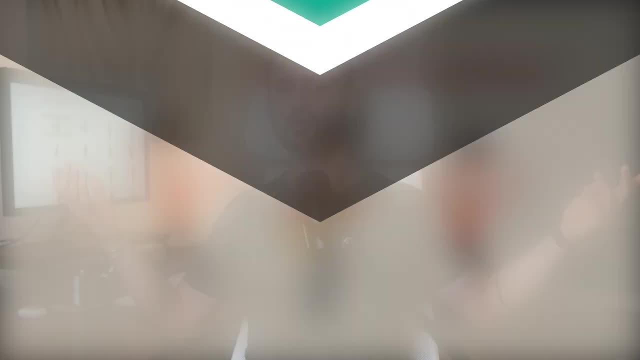 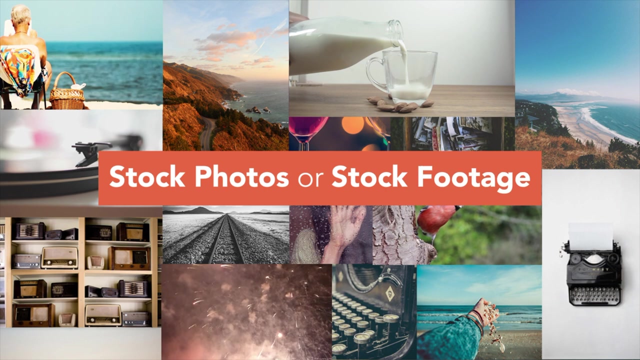 directly in Premiere Pro, then please keep watching, Because I want to introduce you to the concept of stock animation. Now you might be wondering: what is stock animation? It's an animation category in the stock assets industry. So if you've ever heard of or used 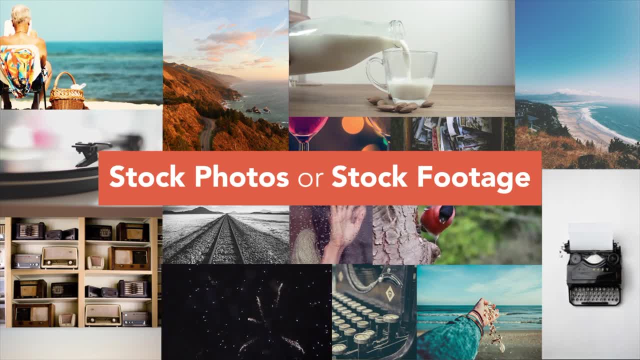 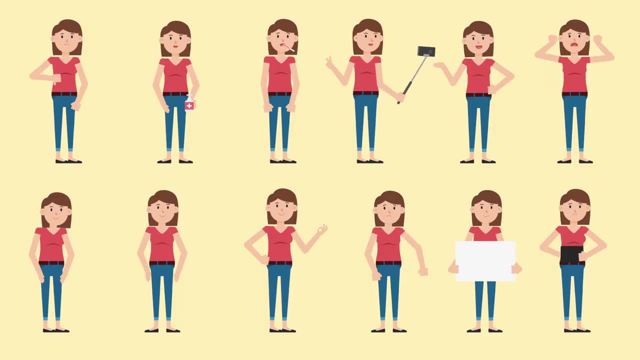 stock videos or stock photos or royalty-free music tracks before. it's literally the same thing, but for animation? If not, let me just explain it real quick. Stock animation videos are basically a library of ready-to-use animated assets that you can purchase and license to use in. 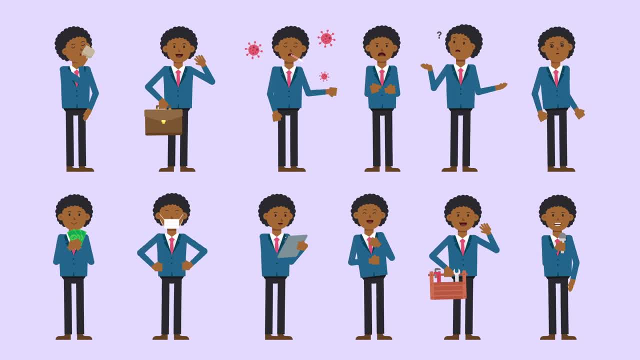 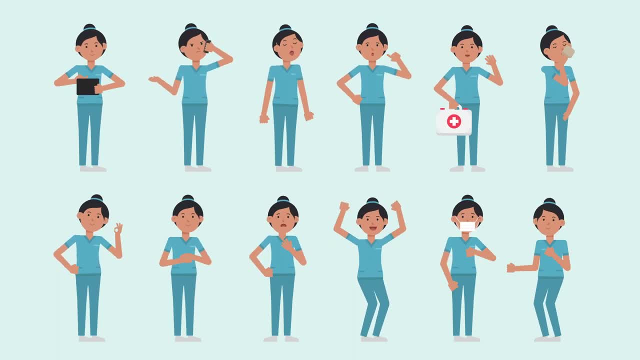 your own video project. They're built by professionals so they look amazing and usually come in sets of characters or icons that you can mix and match to create professionally looking videos with ease. How easy From a technical point of view. the animation is pre-made and 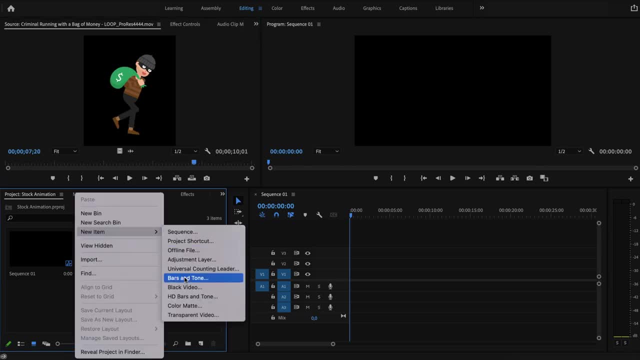 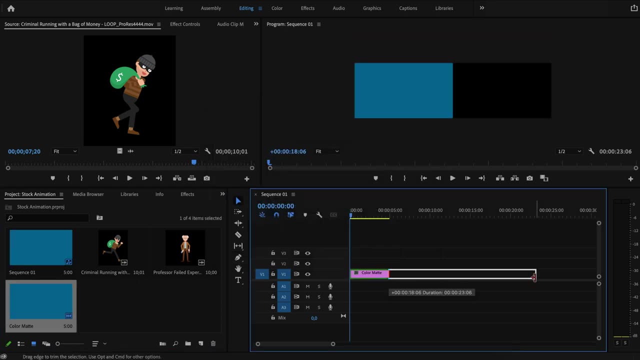 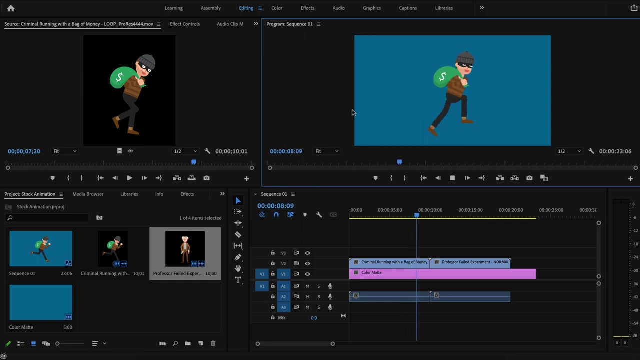 ready to go. All you have to do is import the video file into Premiere Pro by drag and dropping it, in the same way you would import any other media. Then just add it on the timeline and press save. You do not have to do anything else. Of course, you can make the scene look even better. 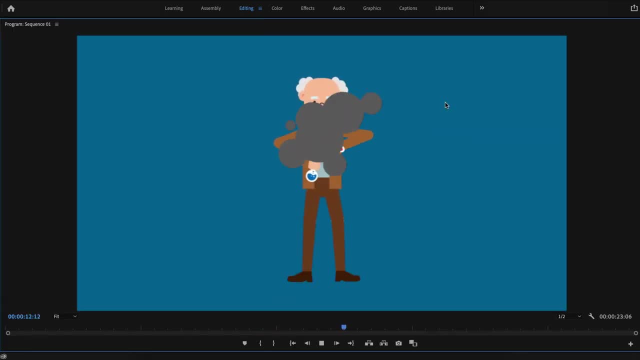 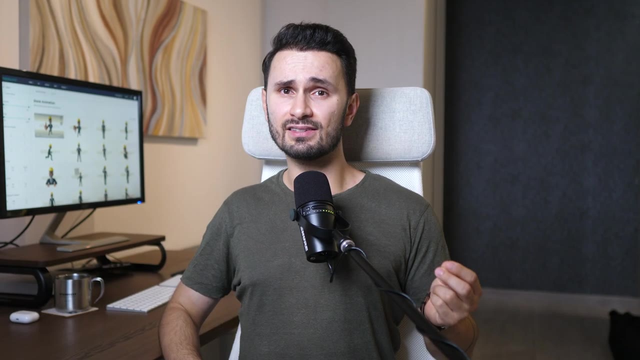 by adding more stock animation elements, changing the background color or adding transitions from Premiere Pro. It doesn't get any easier than that. It now takes you literally minutes to achieve what would otherwise take you tens of hours to produce from scratch. Just find the stock animation videos. 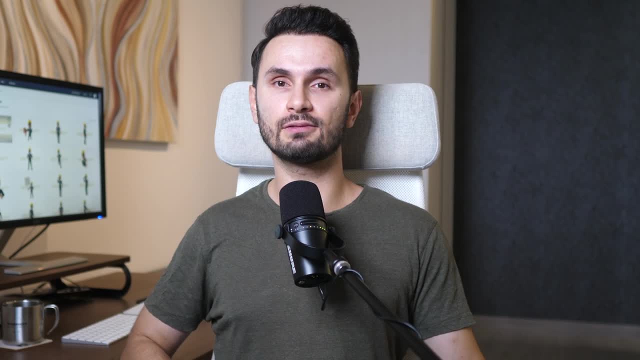 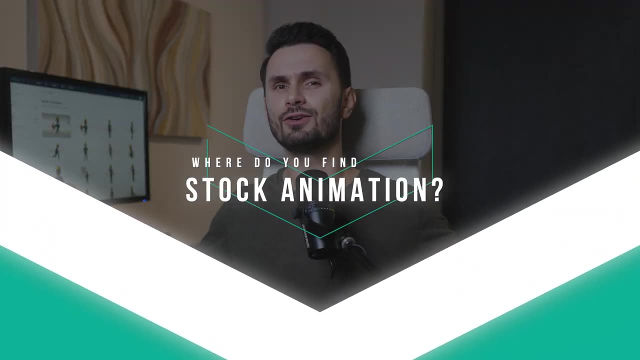 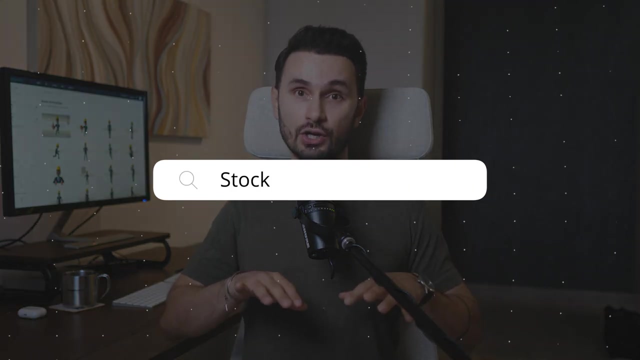 that you need, which work well for your project requirements. download them and add them to your timeline. But now the million dollars. The million dollar question is: where do you find such stock animation clips? Well, one option is to search on Google for stock animation, but the truth is you won't find many. 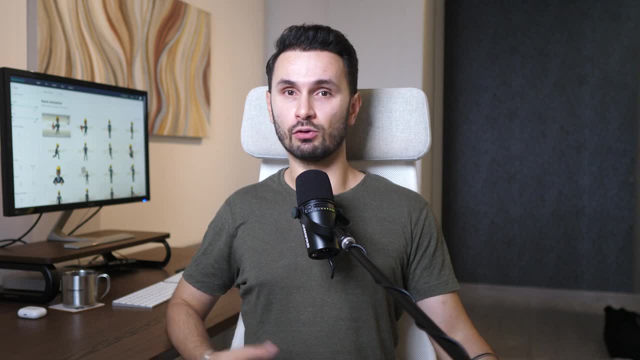 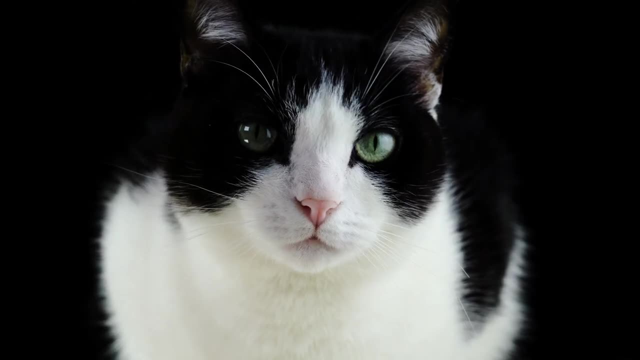 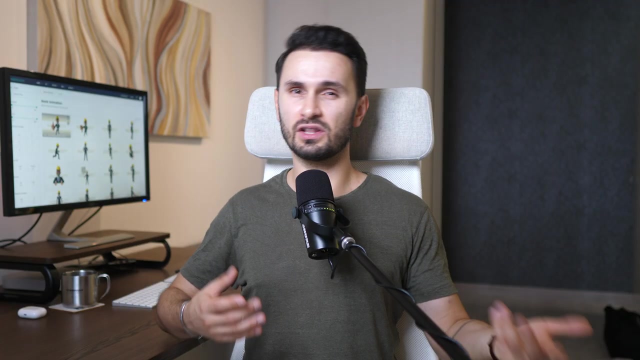 good options. There are some decent clips here and there on stock footage websites, but those websites always specialize in live action videos recorded with cameras, not in animation. So if you ever find any stock animation, it's usually just a bunch of random ones that don't really work. 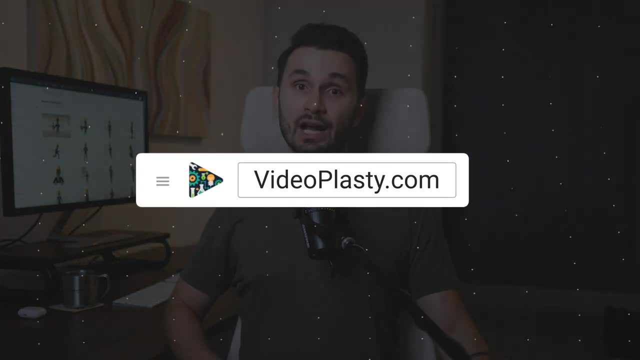 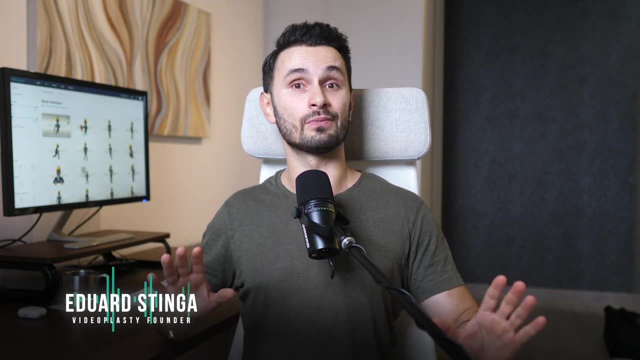 well together. So if you ever find any stock animation, it's usually just a bunch of random ones that don't really work well together. The only good source for stock animation that I know is Videoplastycom. And full disclosure. I'm Eduard Stinga, founder of Videoplasty. Listen, I'm more than happy for. 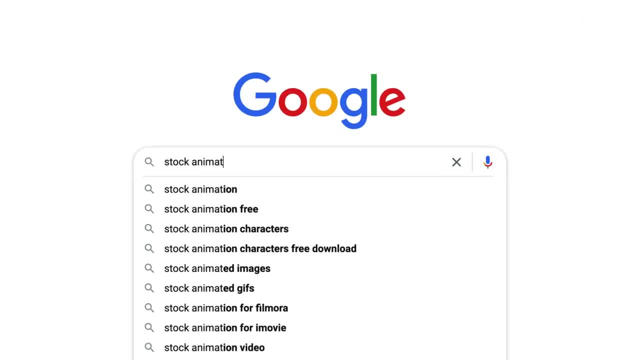 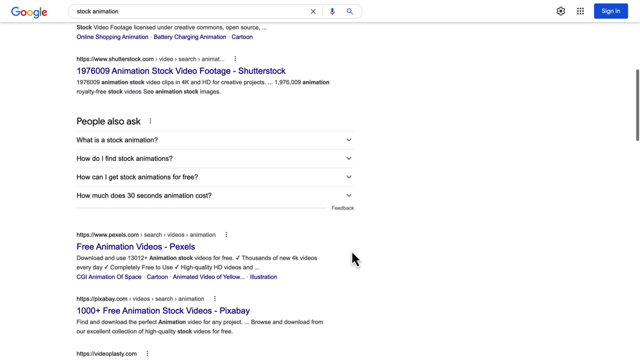 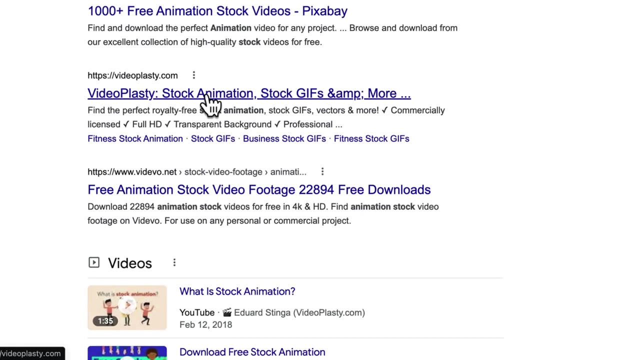 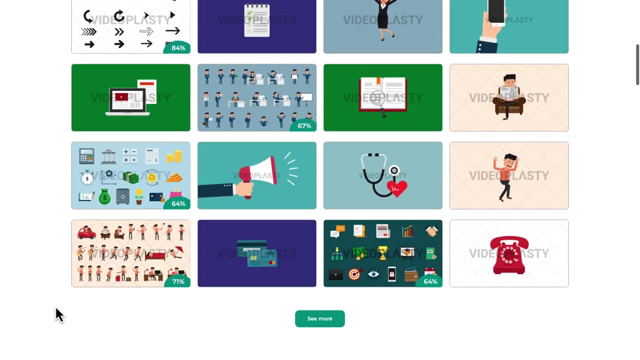 you to look for cool stock animation anywhere else online on other websites, but, honestly, Videoplasty is the only platform in the world dedicated to selling this kind of professionally looking stock animation videos that are available exclusively only on Videoplastycom. So if you are interested to easily create professional animations directly in Premiere Pro, 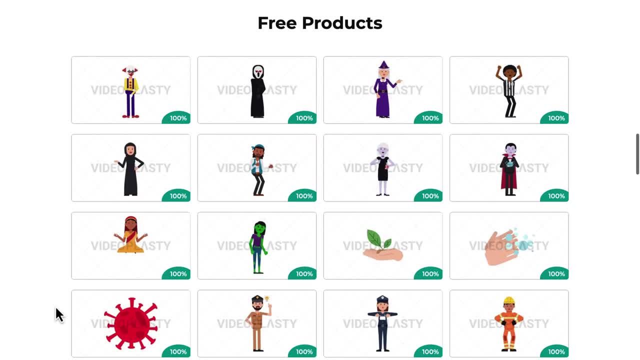 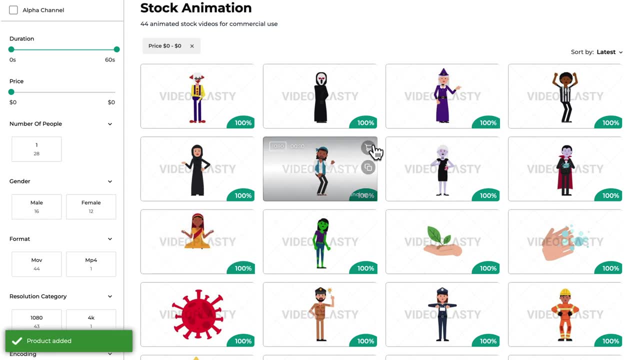 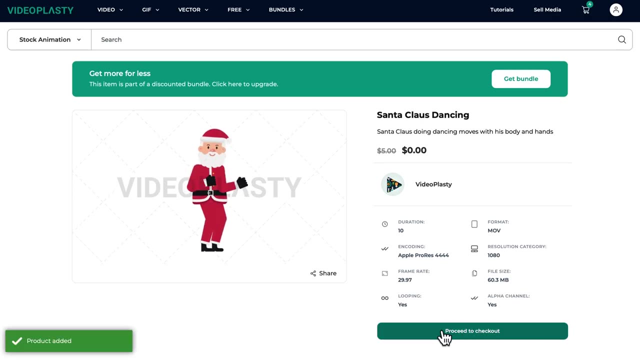 with drag and drop simplicity without wasting countless hours learning new skills. you can literally make cool animations right now. after watching this video, then I highly recommend you check out our website for yourself. We have a free section where you can download a bunch of free stock animation clips to have fun with and see how easy the whole thing is.